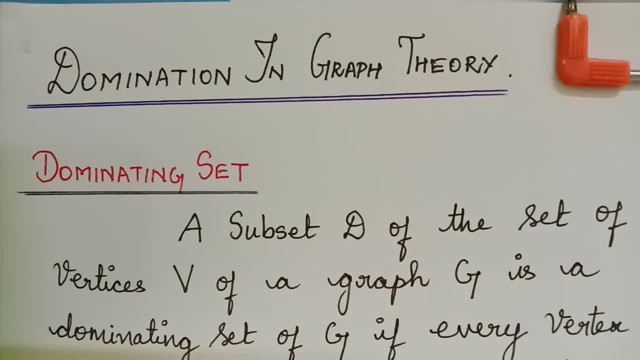 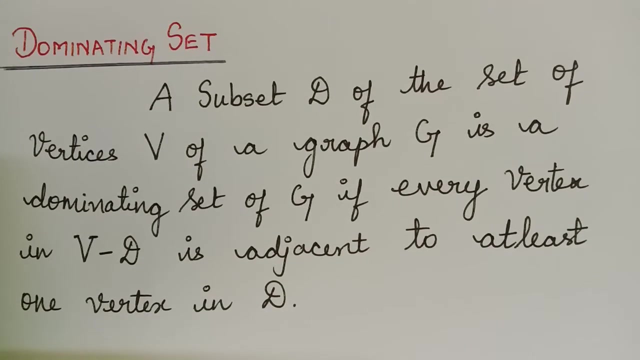 Hello students, in this lecture let us learn about domination in graph theory. The concept of domination in graph theory is a very significant topic. We shall first see the definition of a dominating set. A subset capital D of the set of vertices V of a graph. G is a dominating 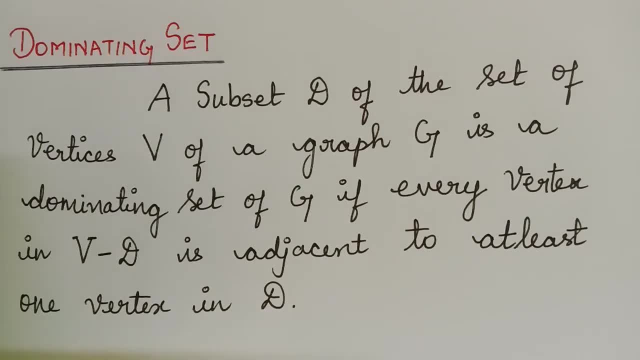 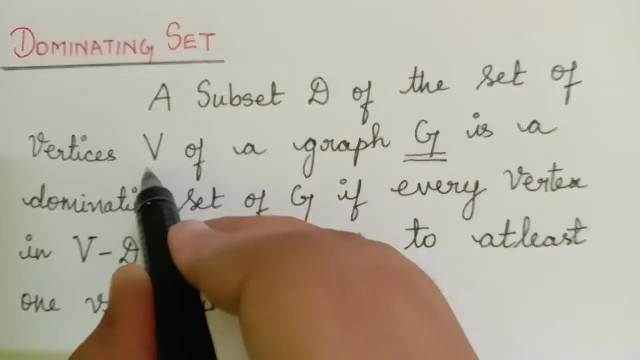 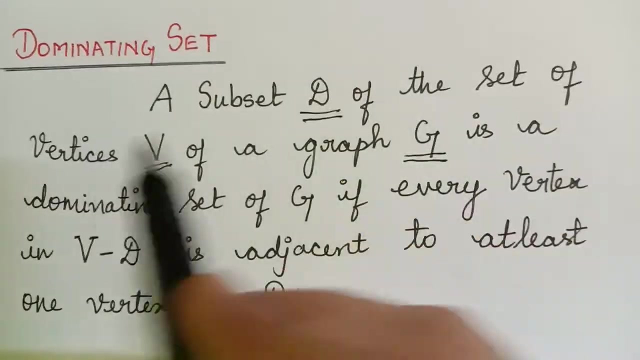 set of G if every vertex in V minus D is adjacent to at least one vertex in D. So first we will consider a graph G with the vertex set V. So a dominating set represented by capital D will be a subset of the vertex set V. So the first condition for a set to 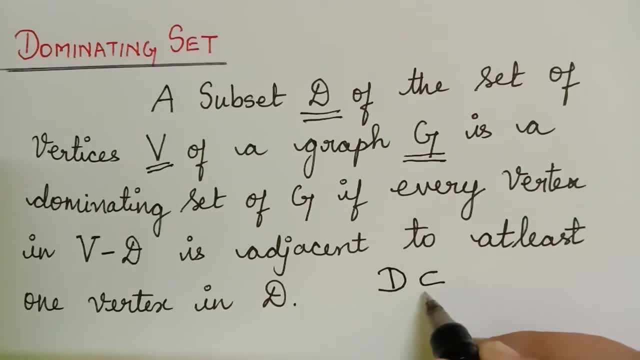 be a dominating set is a subset of the vertex set V. So the first condition for a set to be a dominating set is it has to be a subset of the vertex set V and secondly, every vertex in V minus D. that is, if we remove the set of vertices which is in D from V. So if we remove D from V, 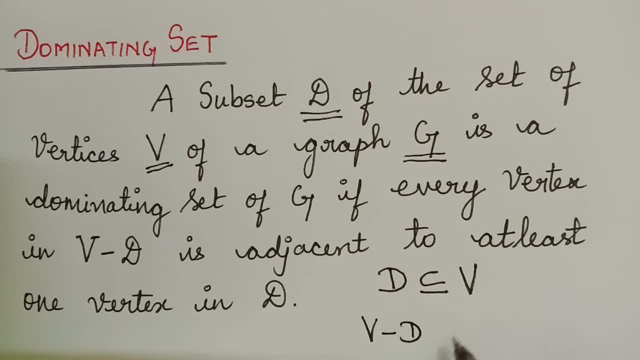 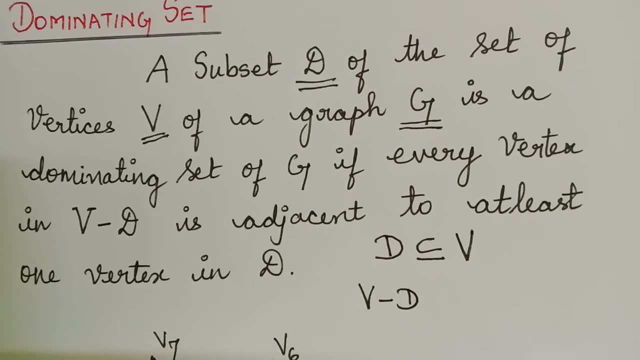 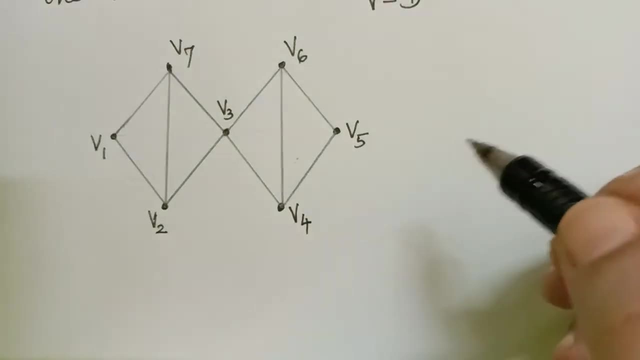 it will be adjacent to at least one vertex in D. So if these two conditions are satisfied, then the set D becomes a dominating set. So if we remove the set of vertices which is in D from V, we shall see this with the help of a graph. We shall consider this graph. Now let us consider: 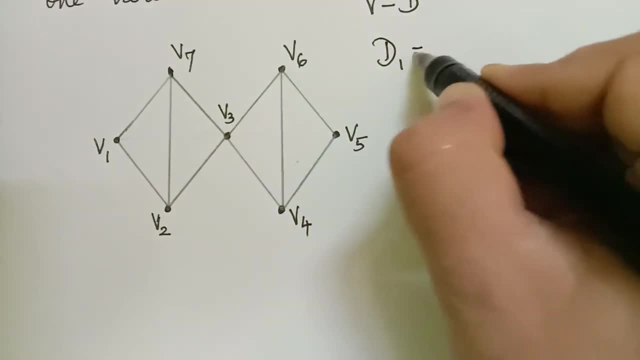 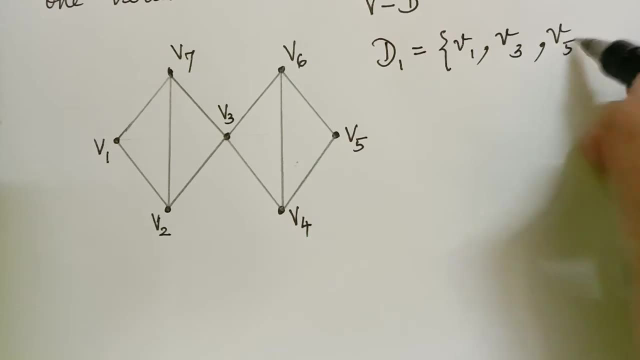 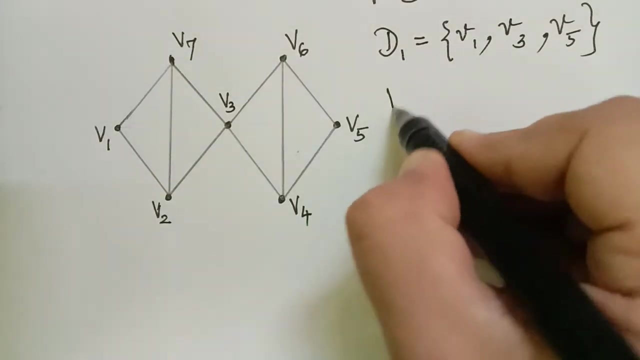 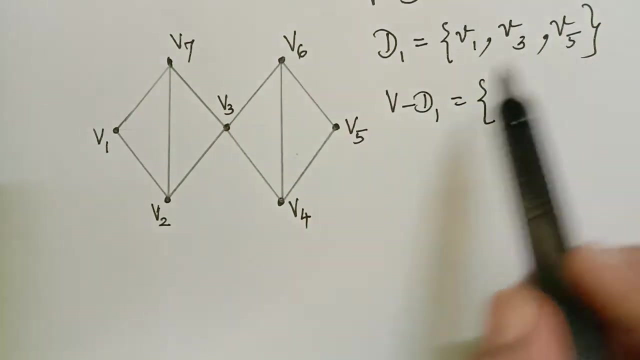 the set D1. So which is equal to V1, V3, V5.. Now let us check whether this is a dominating set or not. So first we have to find V minus D1. So what will be V minus D1.. So if we remove these vertices from the vertex set of G, So that 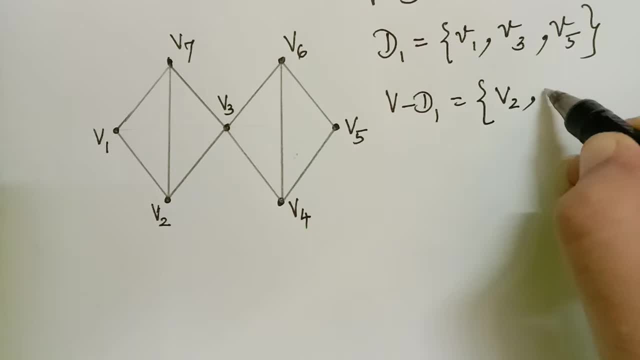 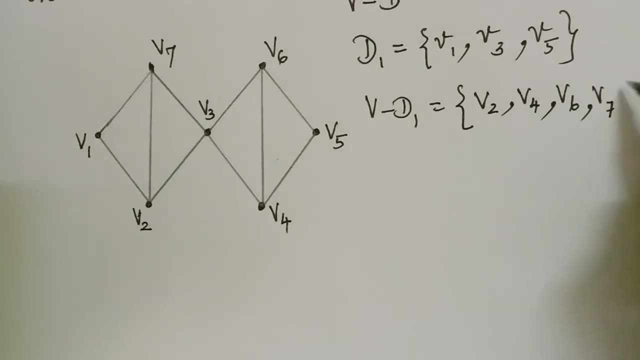 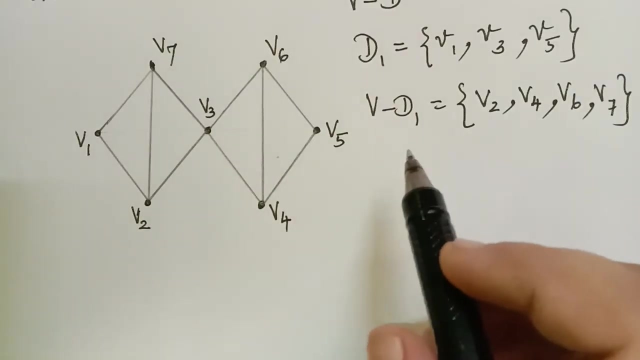 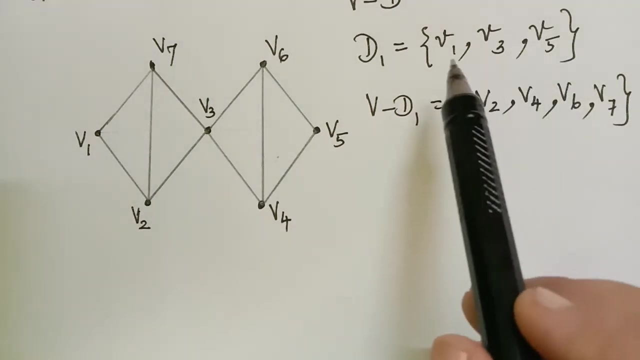 will be V2, V4, V6 and V7.. So these are the vertices of V minus D1.. Now we have to check whether every vertex of V minus D1. is adjacent to at least one vertex in D1. So let us check it now. First we shall consider the 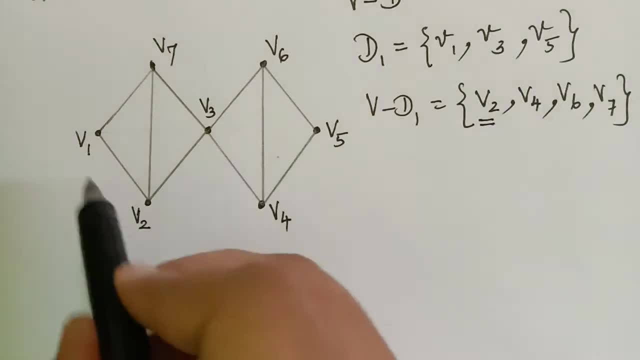 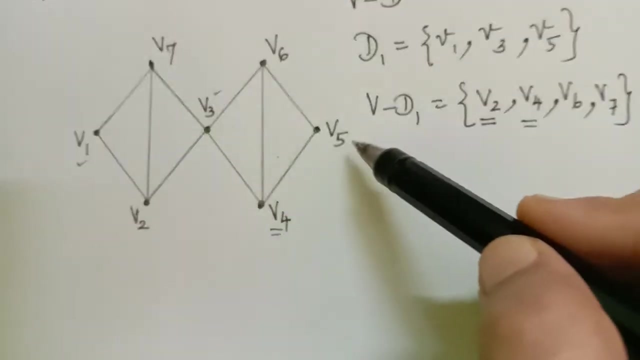 vertex V2.. Now, V2 is adjacent to V1 as well as V3.. So it is adjacent to more than one, of course. So now we shall consider the vertex V4.. The vertex V4 is adjacent to V3 and V5. 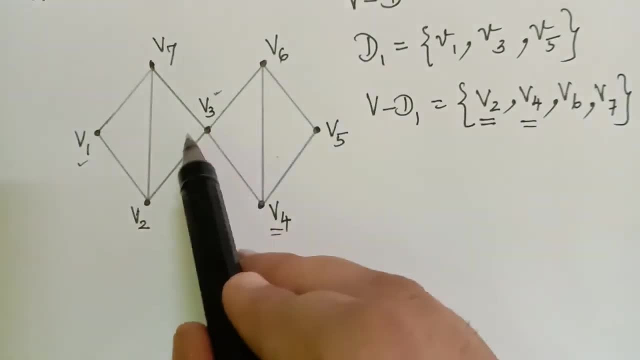 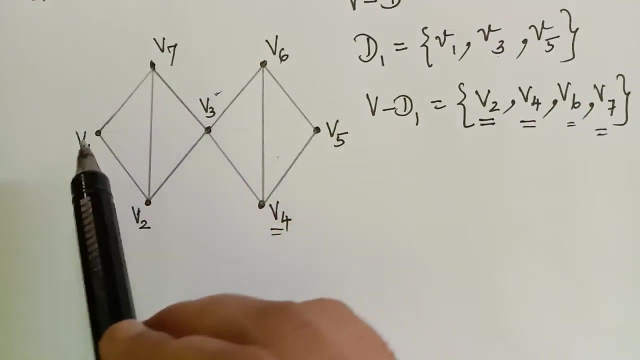 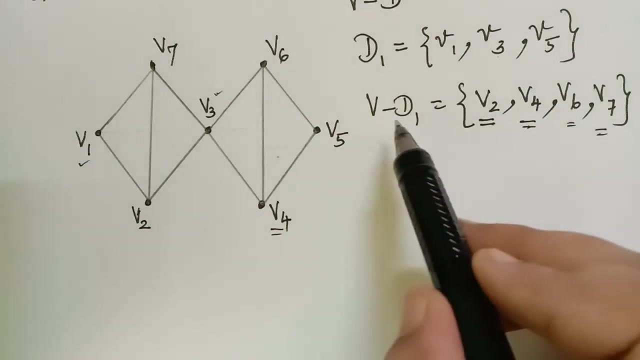 The vertex V6. is adjacent to V3, V5, which is in D1. And also the vertex V7 is adjacent to V1 and V3, which is in D1. So therefore, every vertex of V minus D1 is adjacent to at least one vertex in D, In fact. 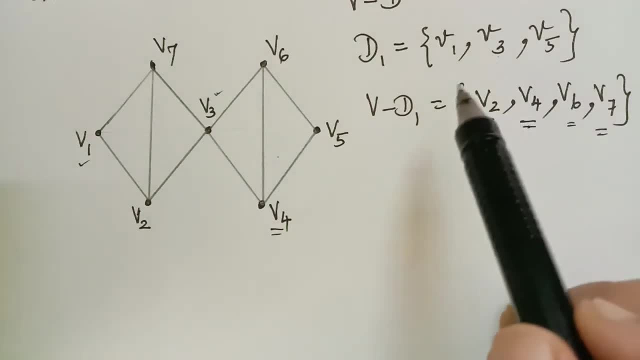 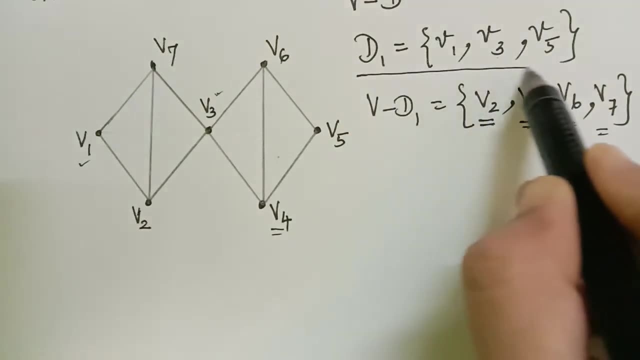 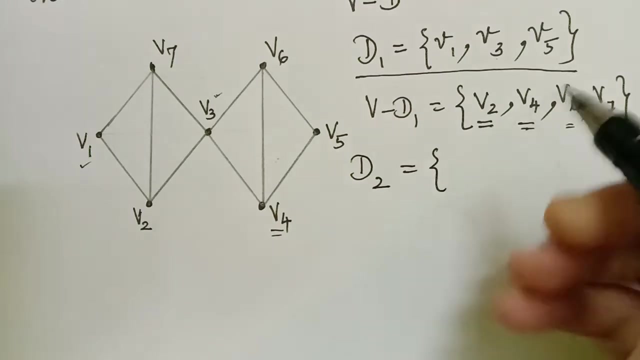 here it was adjacent to more than one vertex. But the main condition is it has to be adjacent to at least one vertex. Then we can say that D1 is a dominating set. Now we shall consider another set, D2.. So let us check whether D2 is. 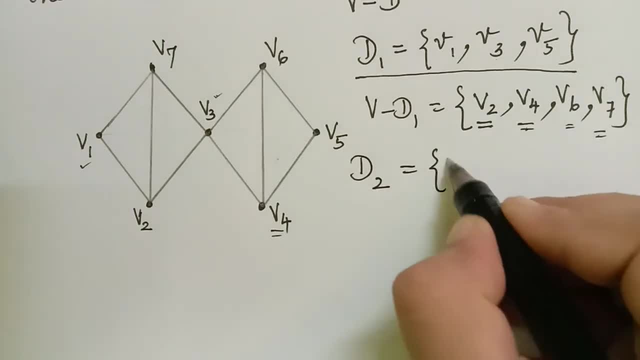 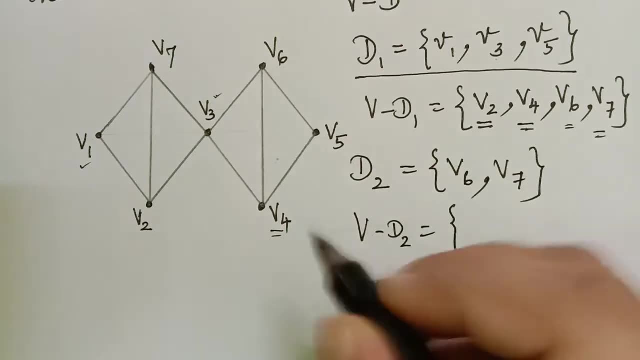 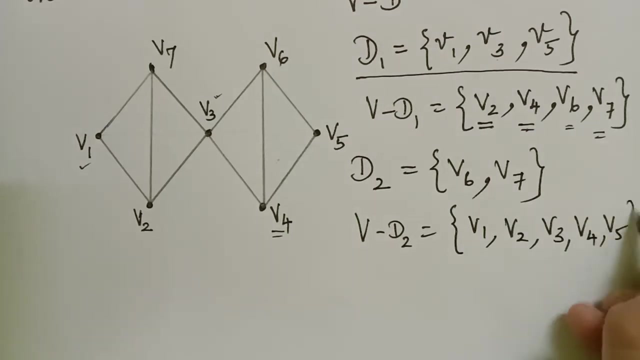 a dominating set or not. The vertices of D2: we will take it as V6 and V7.. So V minus D2 will be the remaining vertices, which is V1, V2, V3, V4 and V5.. Now we shall check whether D2 is a. 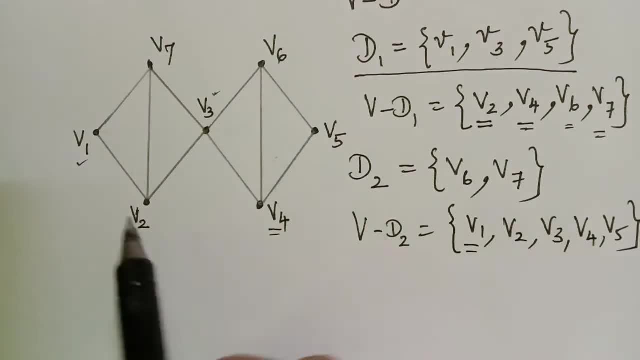 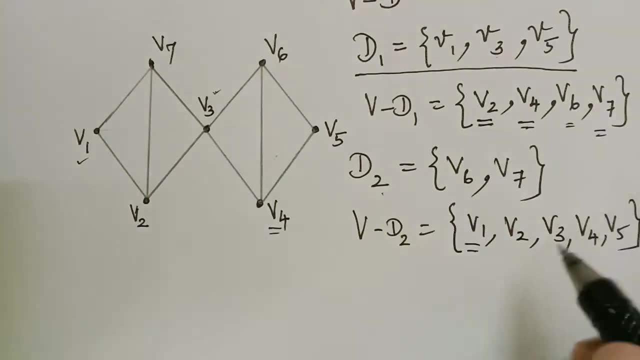 dominating set or not. So when we take V1, so V1 is adjacent to V7. So it is adjacent to V7, which is a vertex of D2.. V2, if we consider again V2, is adjacent to V7. So this is also working out. 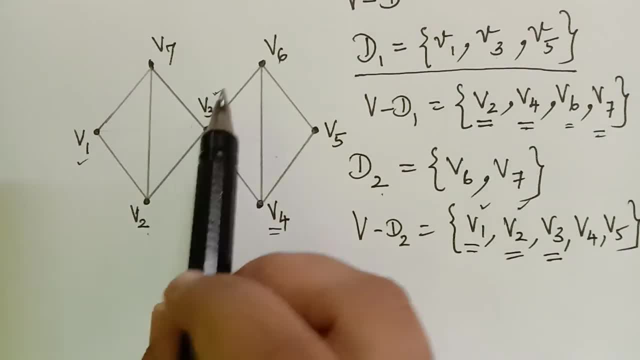 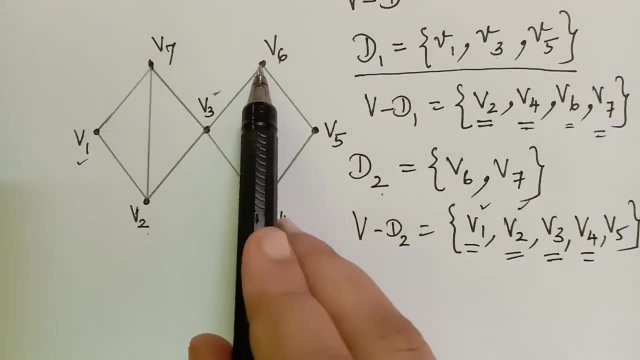 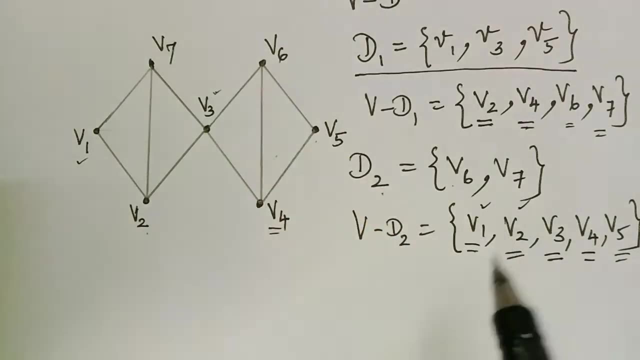 Now V3, when we consider it is here, which is adjacent to both V6 and V7. Then V4, when we take it is adjacent to V6, which is in D2. And V5, when we take it is adjacent to V6. So here also we can. 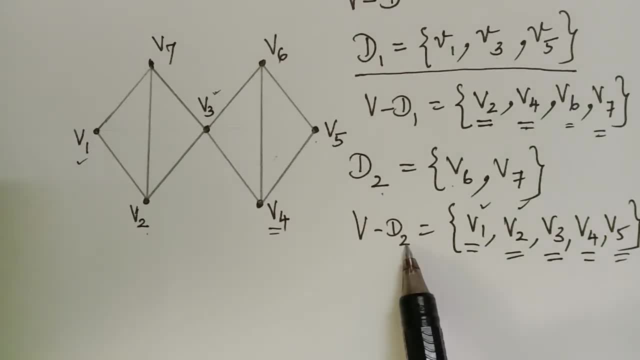 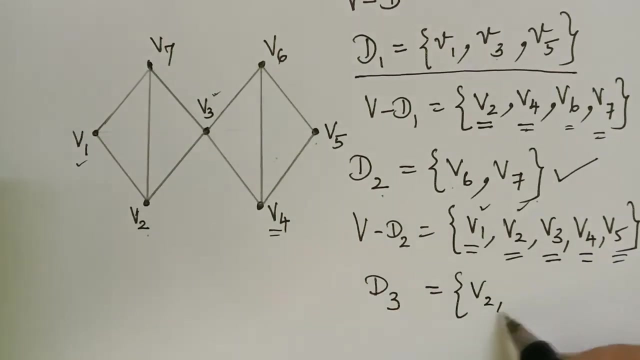 find that every vertex of V minus D2 is adjacent to at least one vertex in D2.. Therefore, D2 is a dominating set. Now we shall consider another set, D3, which is equal to V2,, V3, V4.. Now we shall consider another set, D3, which is equal to V2, V3, V4.. Now we shall consider another set, D3, which is equal to V2,, V3, V4. 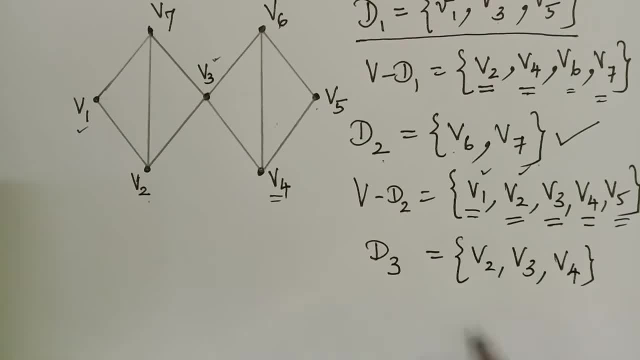 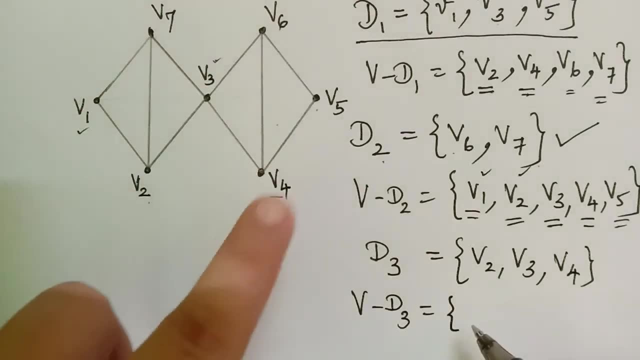 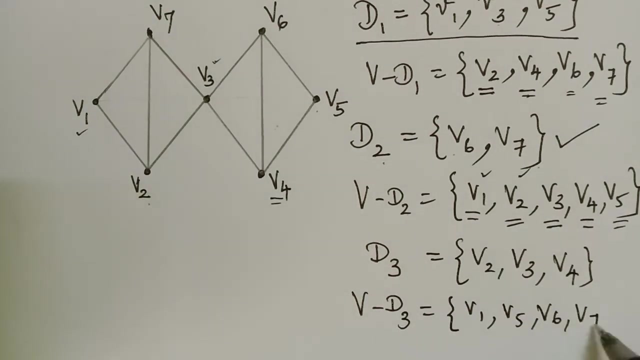 Now we shall check whether D3 is a dominating set or not. So V minus D3 will be equal to. so what are the remaining vertices? after subtracting D3 from V, It is V1, and then V5,, V6 and V7.. 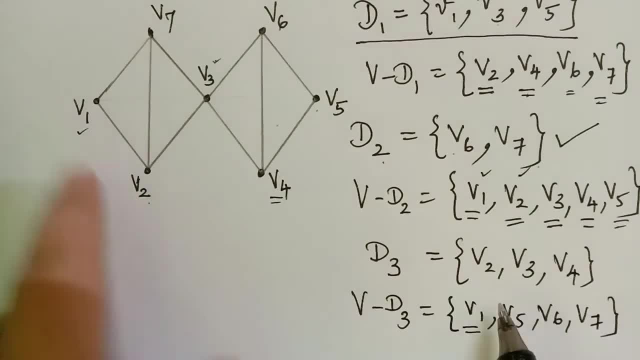 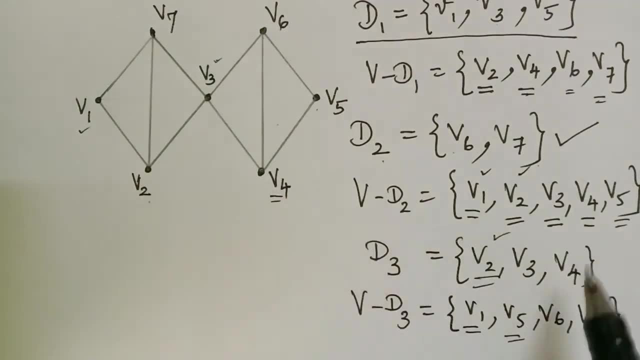 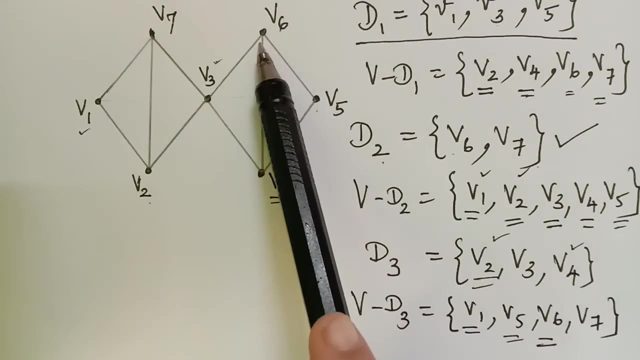 So now, when we take V1, it is adjacent to V2.. Then when we take V5, it is adjacent to V4, which is here. So this is adjacent to one of the vertex of D3. So when we take V6, it is adjacent to V3 and V4 as well. 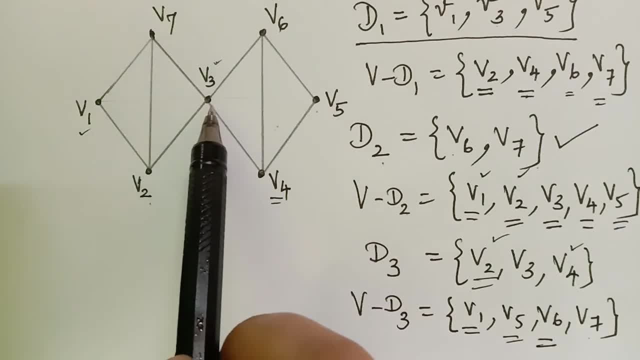 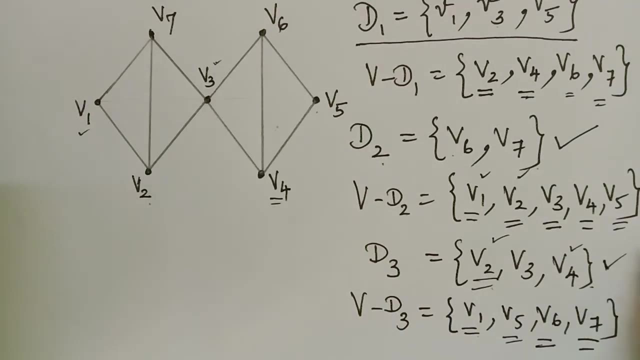 And when we consider V7, it is adjacent to V3 and V2 as well. So all the vertices of V minus D3 is adjacent to at least one vertex of D3. So therefore, D3 is a dominating set. We shall now learn about. 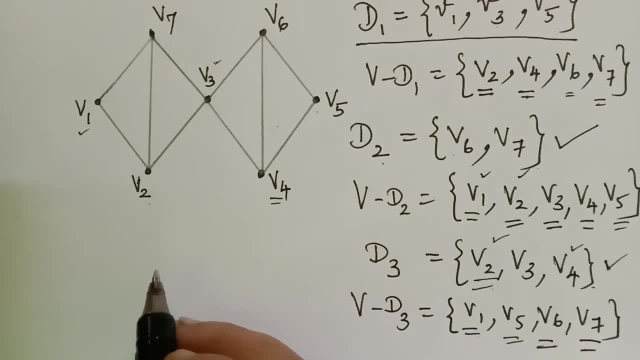 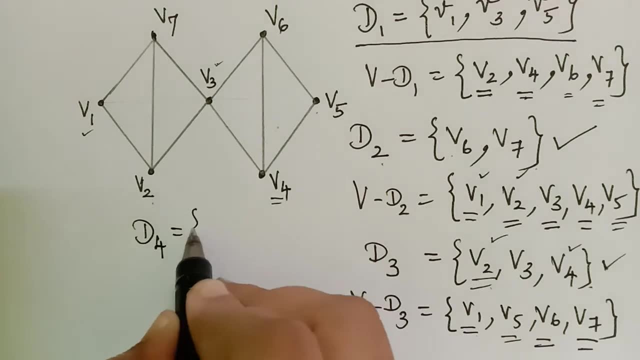 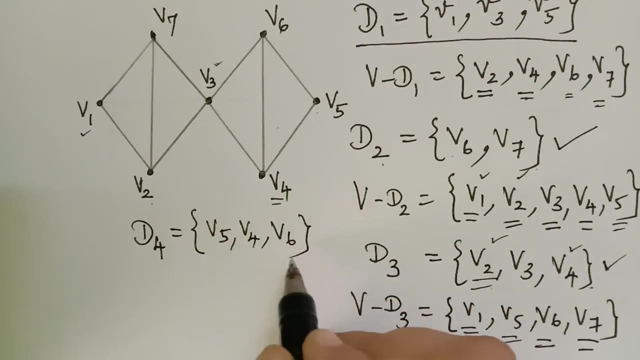 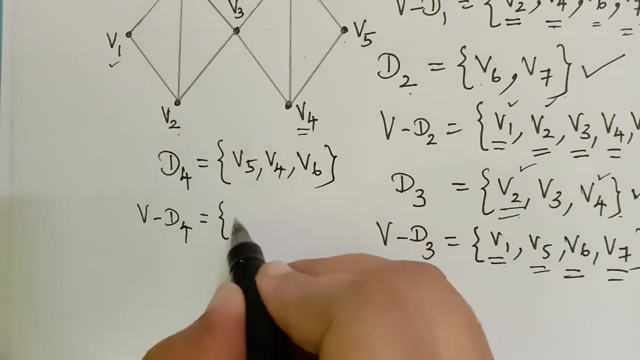 domination number Before learning about it. now we shall see an example of a set which is not a dominating set. For example, we shall consider a set D4, which is V5, V4 and V6. Now, when we take this, we can see that V-D4 will be equal to V1, V2, V3 and V7.. Now, when we check here, 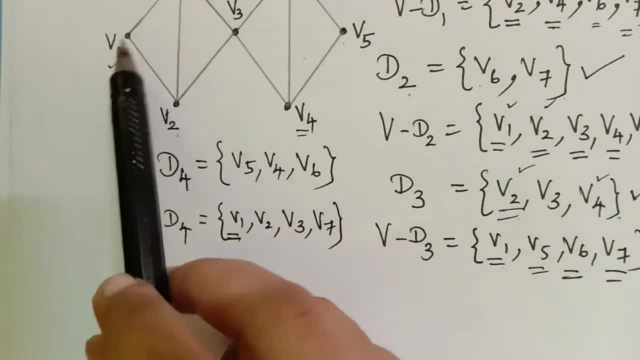 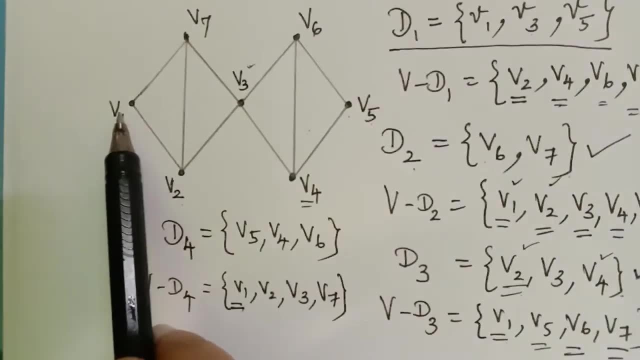 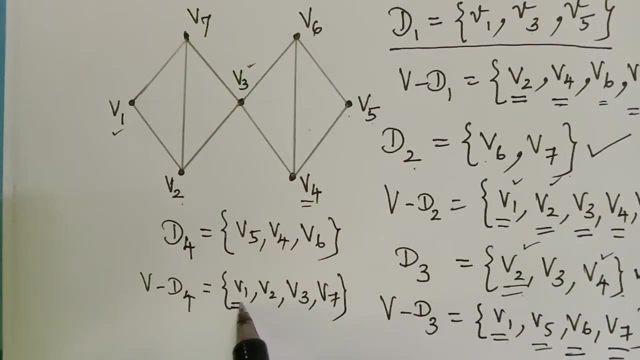 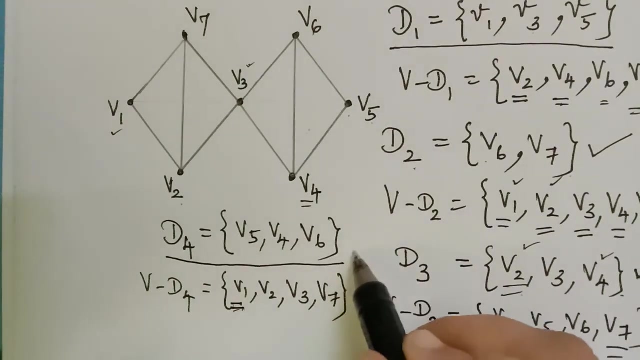 the vertex V1 is adjacent to V7 and V2, only It is not adjacent to V5, it is also not adjacent to V4, neither it is adjacent to V6. So the vertex V1 does not satisfy the condition. So therefore the set D4 is not a dominating set. 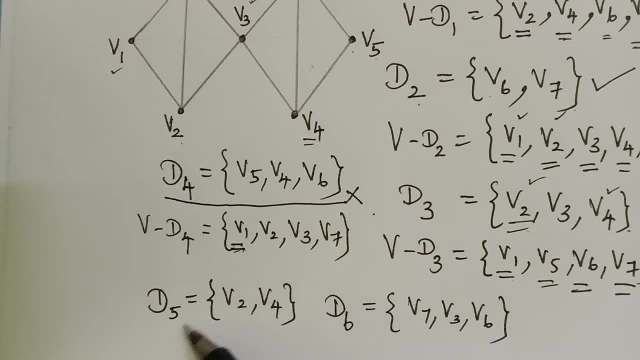 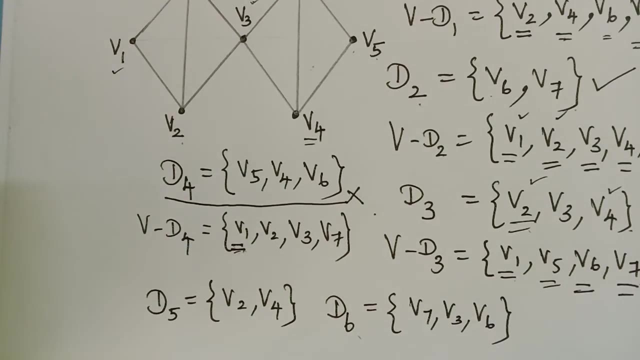 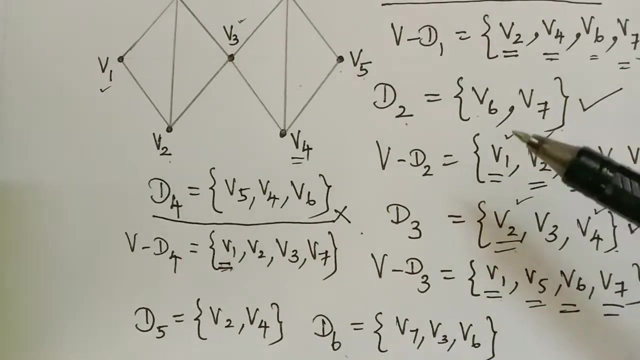 So these are other dominating sets of this graph. Now we shall learn about domination number. For that we should know what is a minimum dominating set. So minimum dominating set, how we have to find, is among the dominating sets, the set which has minimum number of vertices. 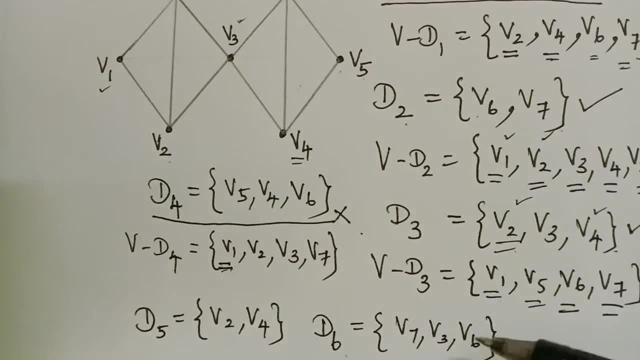 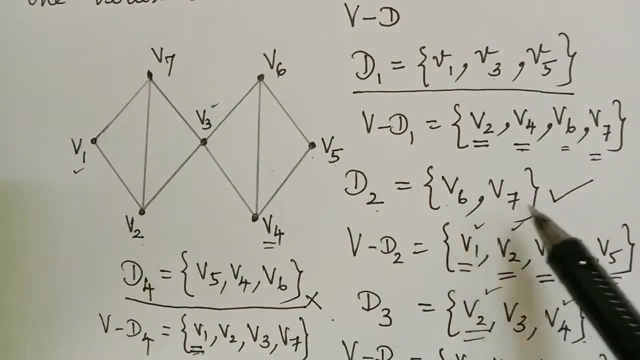 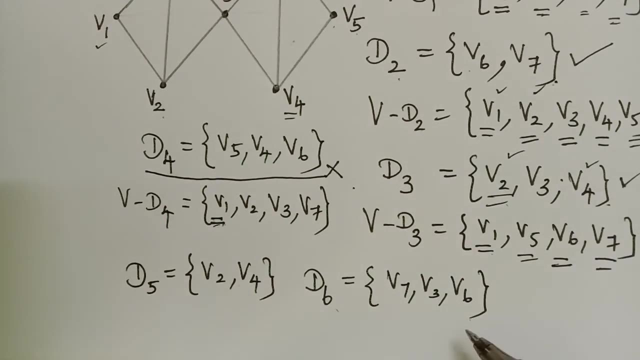 will give us the minimum dominating set. Now, for example, in this graph, the dominating set d1 has 3 vertices, D2 has 2, d3 has 3, and then D5 has 2 and d6 has 3 vertices. Now, if we see, D2 has. 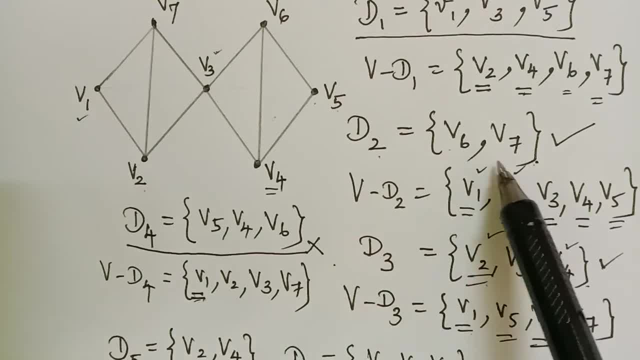 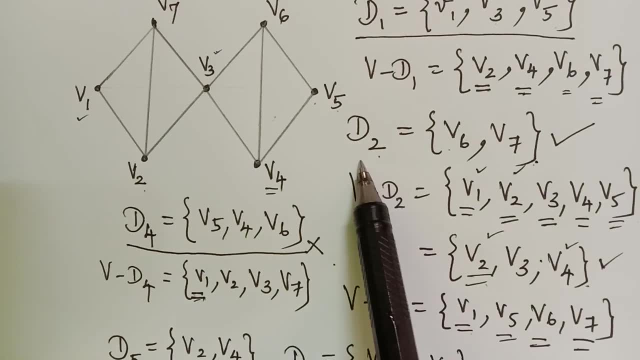 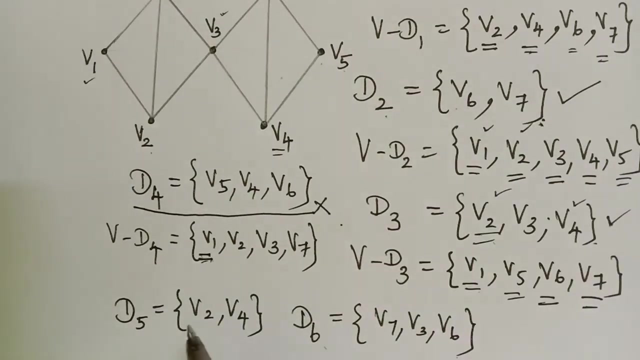 and v7, which is two vertices. Now, if we remove any one vertex from this, this set will lose the property of being a dominating set. Then we cannot have a dominating set lesser than two vertices. So therefore the minimum dominating set is d2 and d5 for this graph. Now the number of vertices: 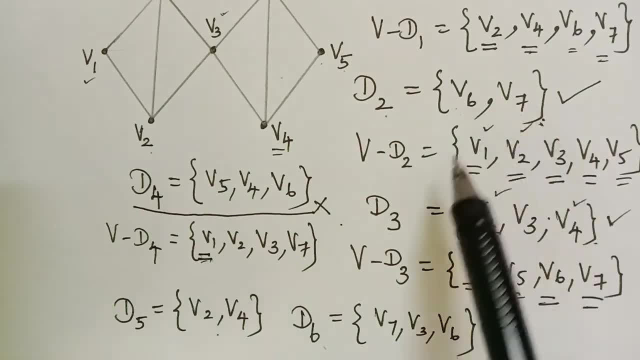 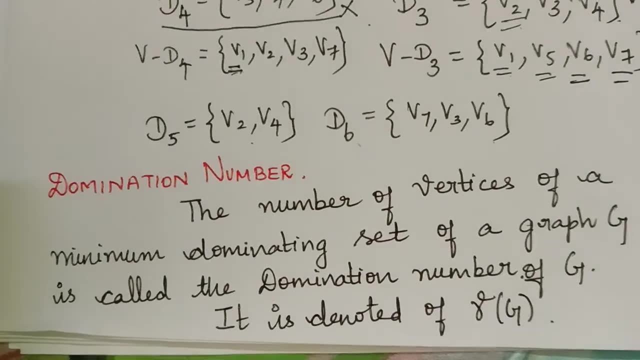 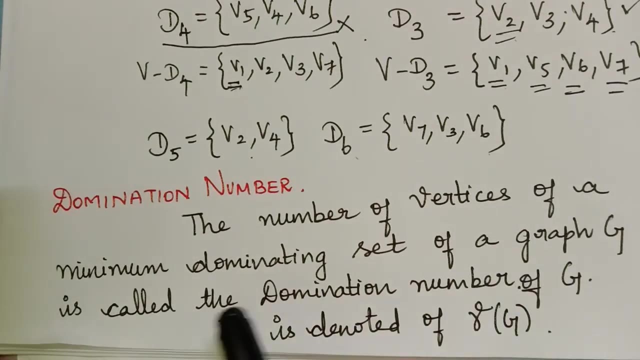 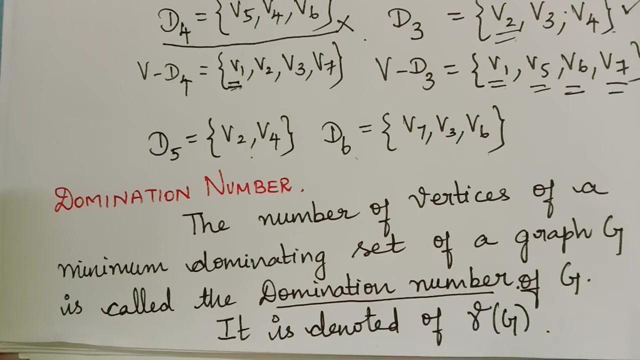 of the minimum dominating set will give us the domination number. So therefore, the definition of domination number is the number of vertices of a minimum dominating set of a graph. g is called the domination number of g. It is represented by gamma of g. So the domination number for this 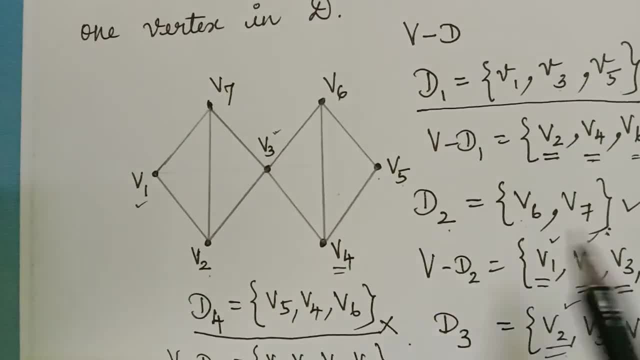 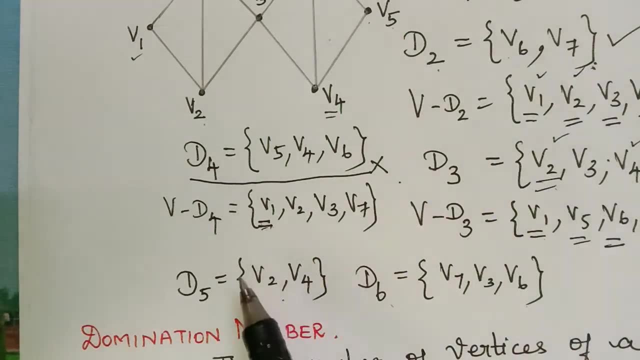 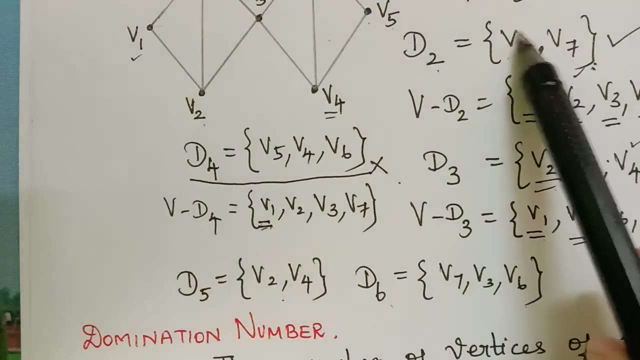 graph will be 2.. As d2 has two vertices and d5 also has two vertices. that is, these two are the minimum dominating set of this graph and the number of vertices of these two, d2 and d5, is 2.. So, therefore, the domination 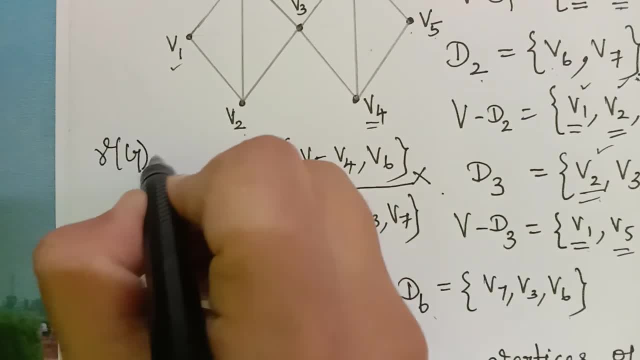 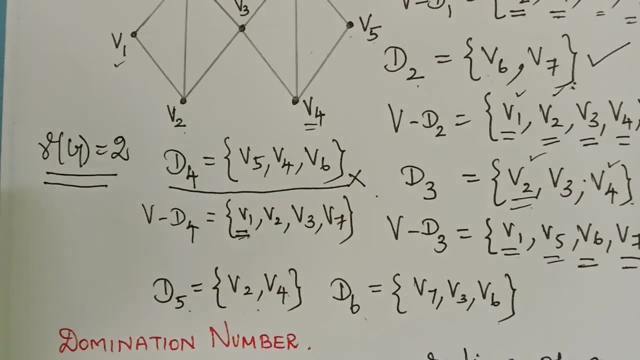 number for this graph is: gamma of g is equal to 2.. Hope you all have understood the concept of domination. Thank you.